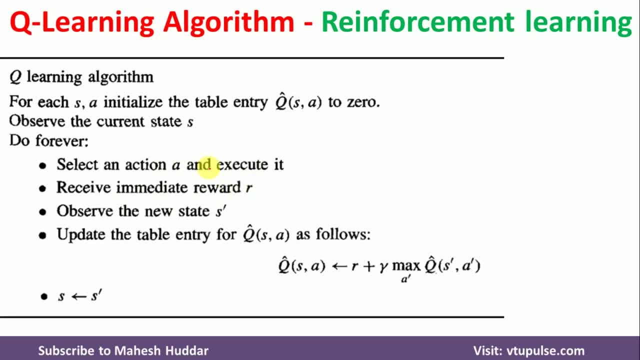 say that particular reward as R in this case. And whenever you perform an action A, you will move from current state yes to a next state. We will say that particular next state as yes dash in this case. Once you perform an action A and received a reward R after that, you will reach. 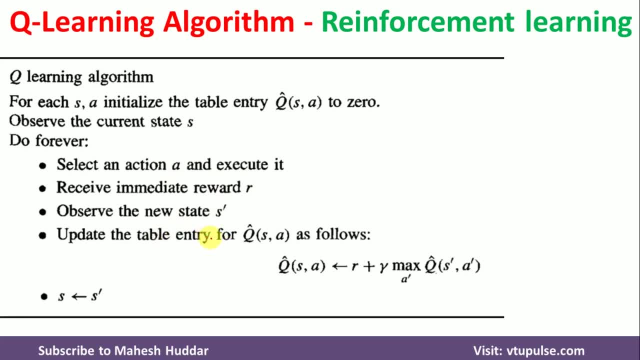 yes, dash. Now you need to update the table entry of Q cap of SA as follows: Q cap of SA is always equivalent to R. that is nothing but the immediate reward plus gamma. that is nothing but the discounted value multiplied by max of Q cap of S. dash, A dash for all A dash. That is nothing. but when you perform an action A. 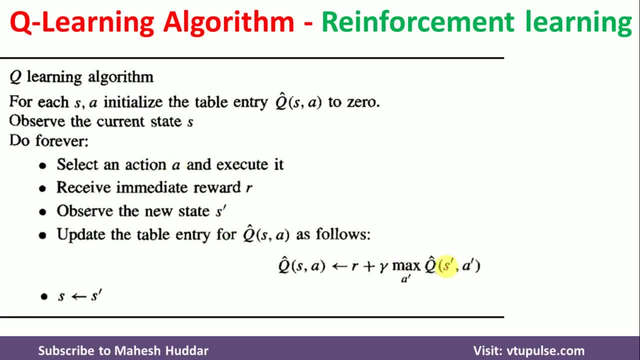 you will move to S dash, that is, the next state, From this particular next state. whatever the actions we can perform, we need to perform those particular actions and then we need to get the immediate reward. The maximum among those things will be the value of this one, And then we need to multiply that maximum value with gamma add it. 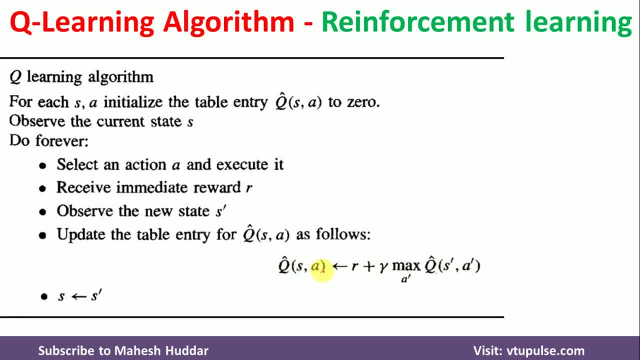 to immediate reward. you will get the updated value for S comma A here Once you perform this particular step. you need to assign this S dash, that is, a new state, to current state. in this case, Once you reach the goal state, you can stop here, Otherwise you need to go back here and then you need to select one action from the S and then execute it, receive the immediate reward. 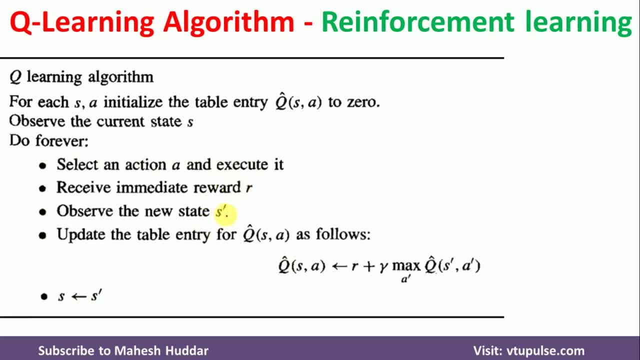 Once you receive the immediate reward, you will get the new state. Once you receive, once you go to the new state, you need to update this particular Q table entry again. The same process is repeated unless and until you reach what you can say that the goal state in this. 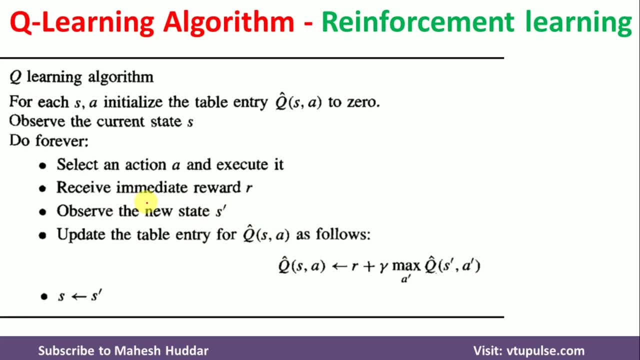 case To understand this particular algorithm better way. I will take one example In the. this is the example I will take In this case. you can see here there are 6, what we can say that the states are there, that is 0,, 1,, 2,, 3,, 4 and 5 and if you want to, 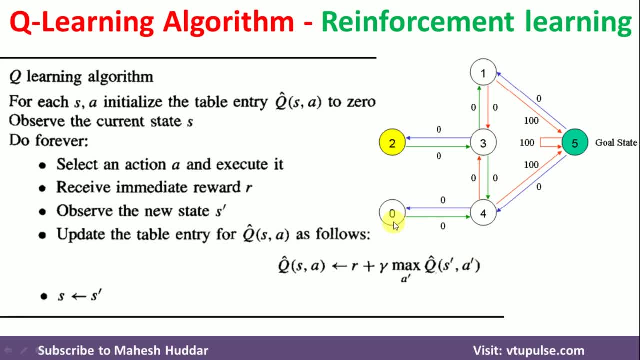 go from one step states to another state. for example, your present at the agent is present in zenoth state and the agent wants to move to fourth state, He has to perform an action. that is this action. the actions are represented with edges, which means that you need to 이걸. 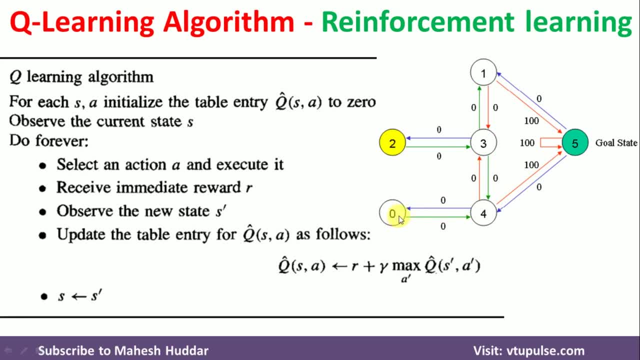 we can give some names or the numbers to that. whenever agent moves from 0 to 4, the action is 4. here, whenever agent moves from 4 to 0, the agent has performed an action of 0. similarly, whenever agent moves from 2 to 3, the action is 3. whenever agent moves from 3 to 2, the action is again you. 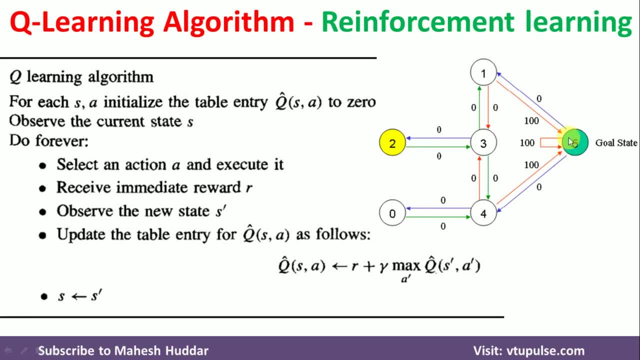 can say that 2 in this case, because 5 is a goal state. in this case, whenever you perform an action and you reach the goal state, the immediate reward will be maximum. in this case, it is 100 here. and one more thing we need to notice here: we need one gamma value, that is, the discounted value. 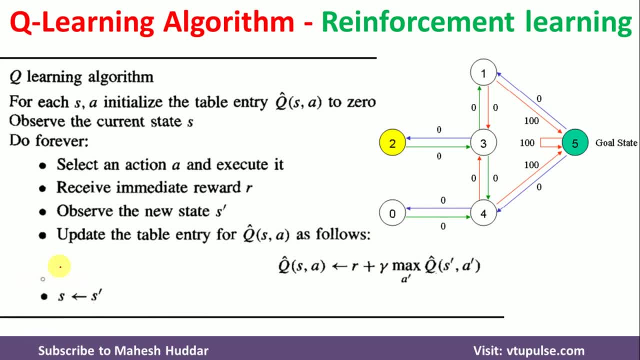 so that we will set it to 0.8 in this case. okay, so first of all i will write gamma here, and then i will have the value as 0.8. now, as per this particular algorithm is concerned, we have two things. one is called as s and a s is a set of state. 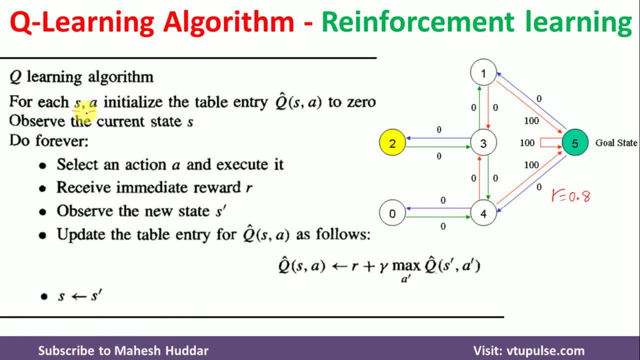 a is a set of actions. in this case we have states like 0, 1, 2, 3, 4, 5. actions are again 0, 1, 2, 3, 4, 5. here now we have to select or observe a current state. assume that i will select this particular state. 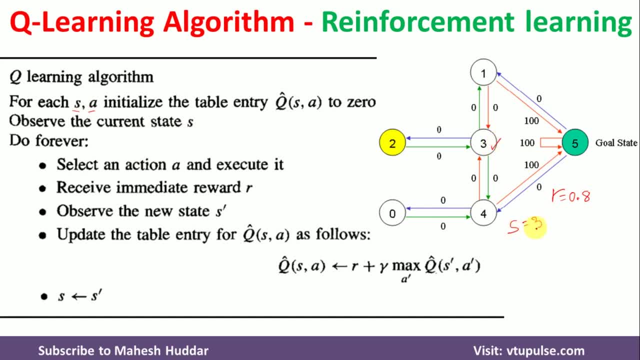 that is 3.. if that is the case, s will become 3. in this case, whenever i am present in this particular current state, i have to perform these particular actions or the steps. this is starting from here: all these particular steps i have to perform unless and until i reach the goal state. so what is the first thing i need to do? 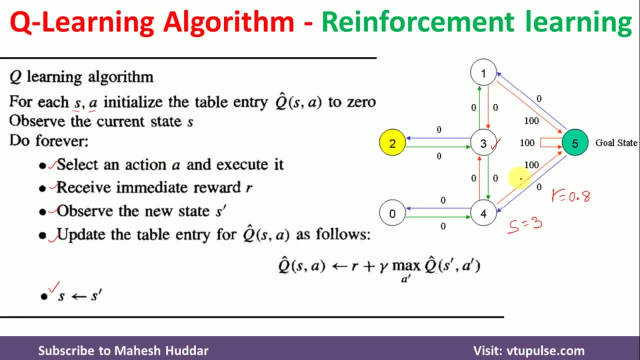 select an action a and execute it. what are the different actions we can perform? first of all, when we are present in state 3, that is, we can perform action 2, 1, 4, that is, i can perform 2, i will go to 2, i will perform 1, i will go to 1, i will perform action 4, i will go to 4.. let us 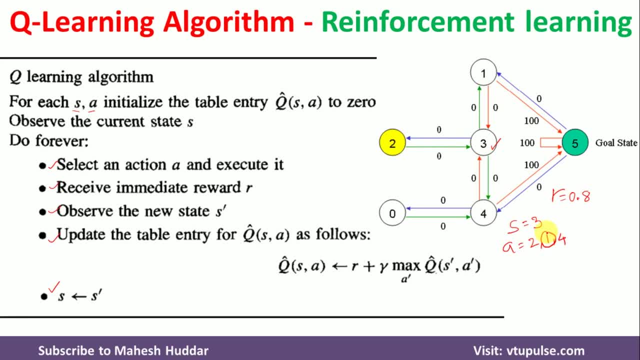 assume that among these three i will select an action- four here, one here, randomly you can select anything. for time being i will select one. now, if i select this particular one, what will happen is i will get an immediate reward, that is, if i perform an action one, i will go to one. so immediate reward is how much? 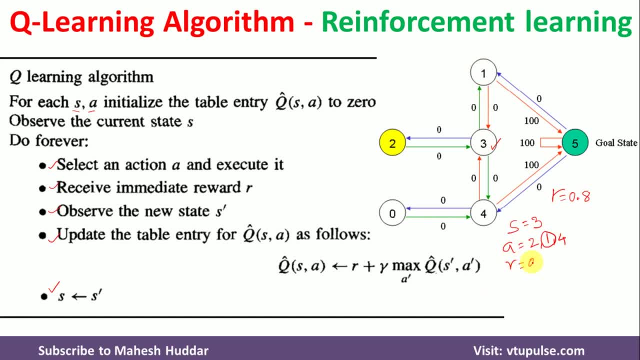 zero here, so r is equivalent to zero in this case. now, whenever i perform this action, i will go to one, so that's the reason s dash will become 1 in this case. now, current state is 3, the next state is 1.. is zero, the action performed is one, so i will put everything in this particular equation here. 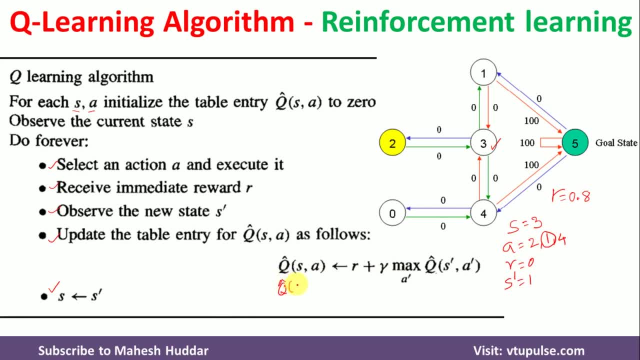 this will become: uh, you can say that q, cap of 3 comma 1, because 3 is the current state, 1 is the action i have selected. immediate reward is three, zero. in this case, uh, plus gamma is 0.08, and then max of q cap of s dash: a dash, s dash is what? 1.. so what are the different actions we can? 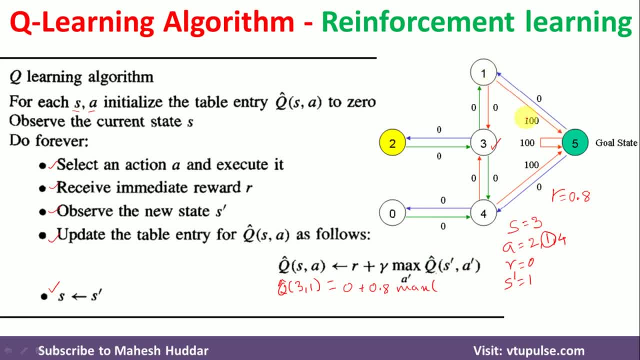 perform. when i am present in one, i can perform. i am present in 1. i can perform different actions. i am present in 1.. I can perform an action 5 or I can perform an action 3 in this case. so whenever I perform action 3, I will get immediate reward of 0. whenever I perform action 5, I will get immediate reward of. 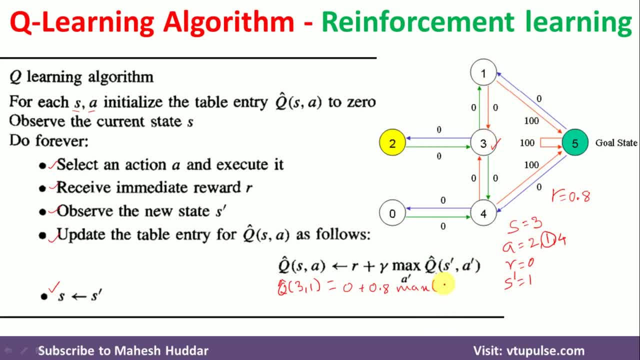 100 here, so between these two, 100 is maximum. so first I will write 0 here, 100 between these two, 100 is maximum. so 100 into 0.8 is equivalent to 80 in this case. so I will get the value for this. 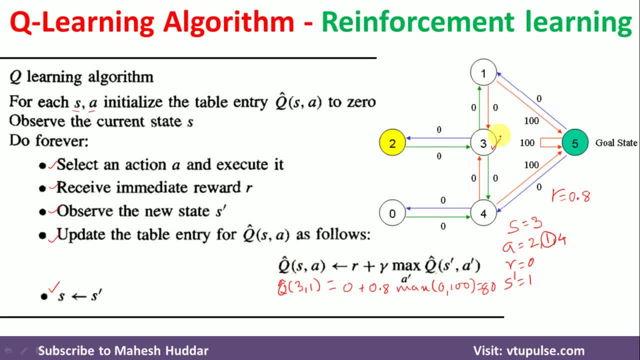 particular current state and the action is 80. that is, the current state is 3 and action is 1, so I will get 80 as the value in this case. now I am present in state 1. that is s dash, so s will become what, according to this particular step. s is equivalent to 1 in this case. now, this 1 is not. 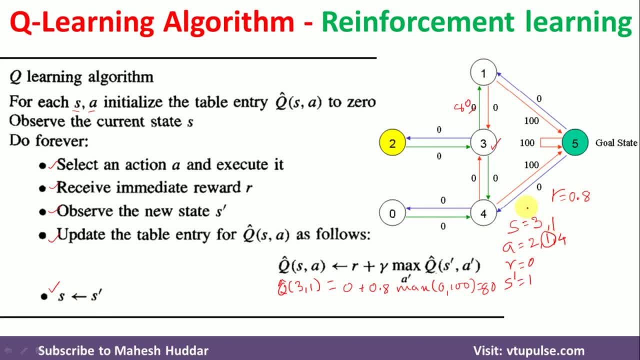 a goal state, so we have to consider this as a current state and then we need to perform unless and until I reach the goal state here. so you, because I am present at state 1, I have to see what all actions I can perform. I can perform an. 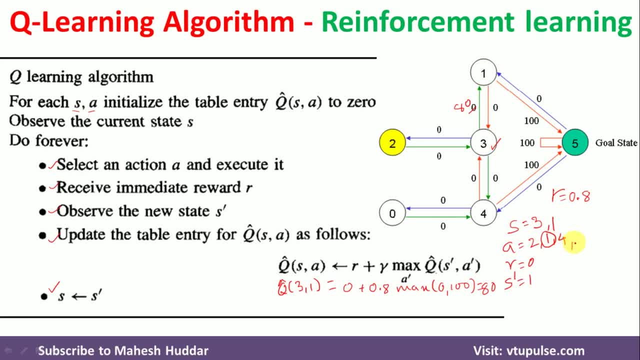 action 5 or I can perform an action 3 here. so 3 is the one action and 5 is the another action. between these two I will select. assume that I will select 5 as the action. if I select 5 as the action, I will get immediate reward of 100 here. so I will put 100 as the immediate reward now if I 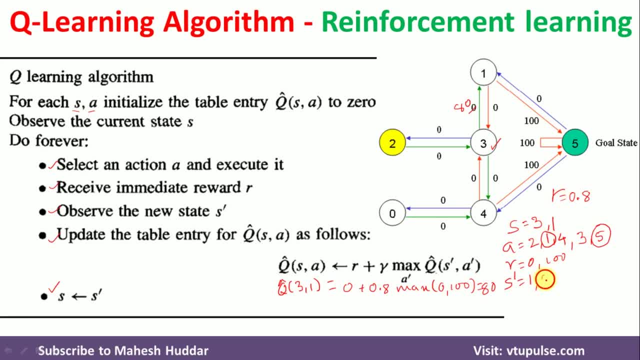 perform this action 5, where I will go. I will go to. the next state is 5 here, so I will go to the complain state where I will put it as 5 in this case. so the current state is 1, immediate reward is 100, the action performed is 5 and I have reached 5, so I will put everything in this. 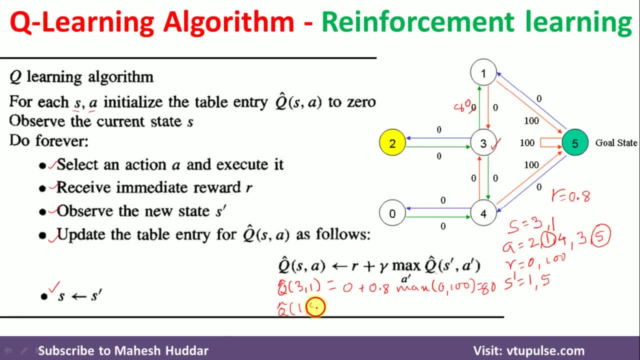 particular equation, that is q camp. it is one. action performed is five. immediate reward is hundred in this case. point eight is the gamma value max of yes s dash a dash. yes s dash is 5. and what all actions I can for form is: I can perform an action one so that I will go to 1, that is the scolding and coming from the acting factor and the action lies in 3 here. so s dash five by after that s dash means gerçekten end of 1. what all actions I can perform is: I can perform an action rokuon desired. the action is two, in which Committee 1 is 0, 0 and 4, in which Q cap. 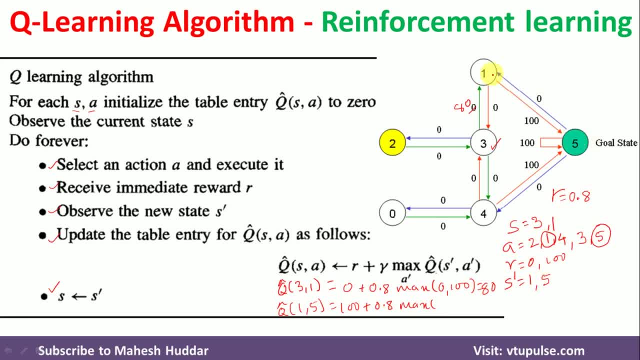 all actions i can perform is: i can perform an action one, so that i will go to one. similarly, i can perform an action four, so that i will go to four. in both the cases i have zero, zero as the value, so maximum between these two zeros is zero, so i will get hundred as the value in this case. 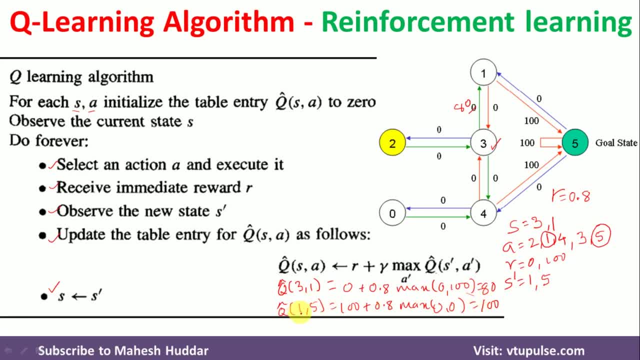 that is uh from five one to five. that is nothing, but i have uh in state one. i have performed an action five and the value for this particular entry is hundred. in this case it is already present here, so there is no need to modify. if there is any change, we need to modify that. 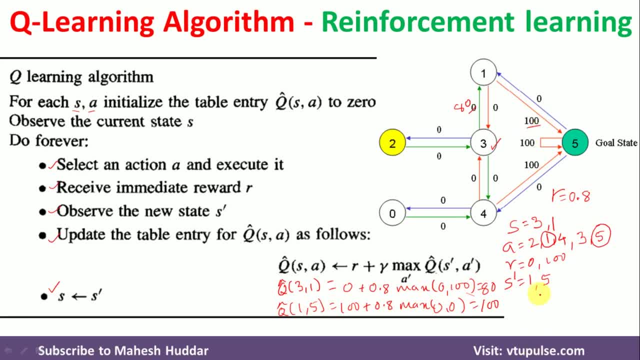 particular value here. now uh s dash is put into yes, so we got five in this particular yes. the meaning of this particular thing is: i have reached the goal state, so one episode has completed. the same process has to be: uh come continued unless and until we remove these particular zeros from. 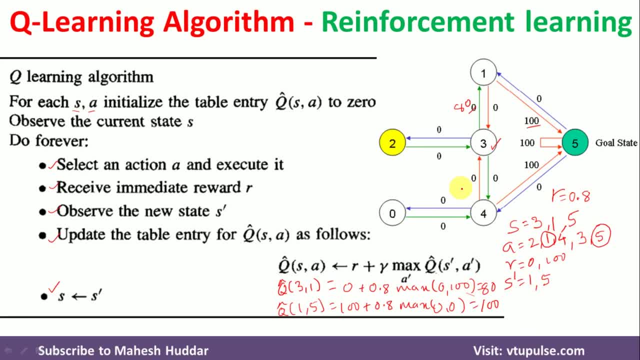 this particular uh, all all the actions over here, uh, that is nothing but uh, considering the different uh state as a current state and then selecting all possible actions and then doing it again and again. once i do this particular thing again and again, definitely i will get the converged values. that is nothing but the final what we can say. that the policy. 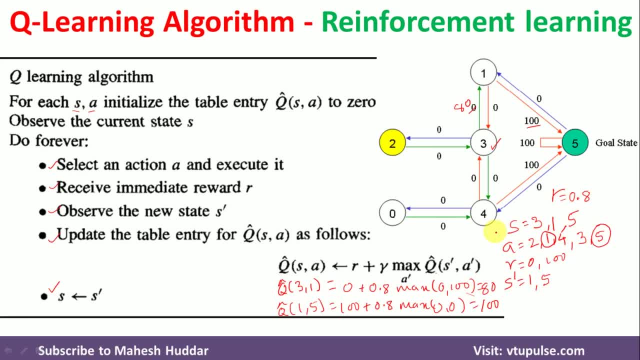 what we have learned in this case. so this is a very simple example so that you can understand how the queue learning algorithm works. in the next video i will consider the same example one more time and then i will try to solve it completely. that is for each and every age. i will try to.